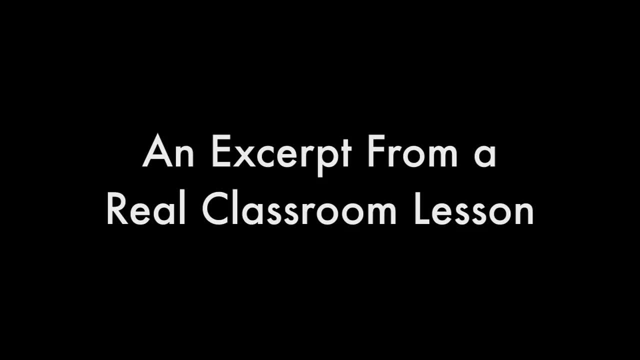 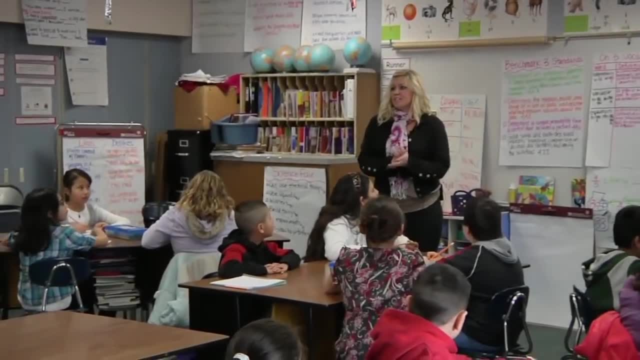 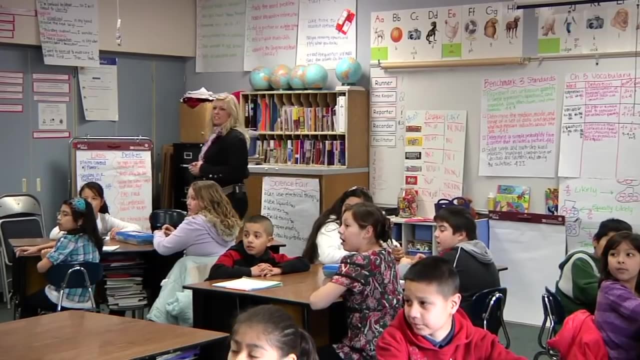 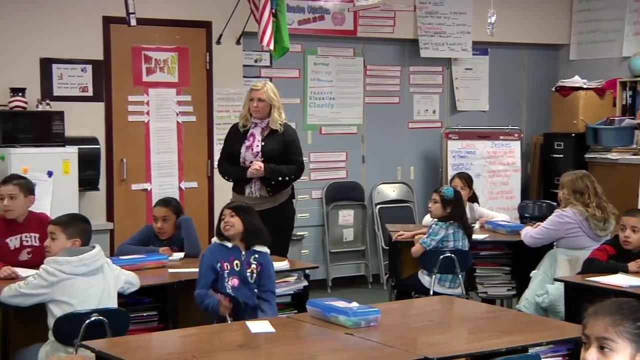 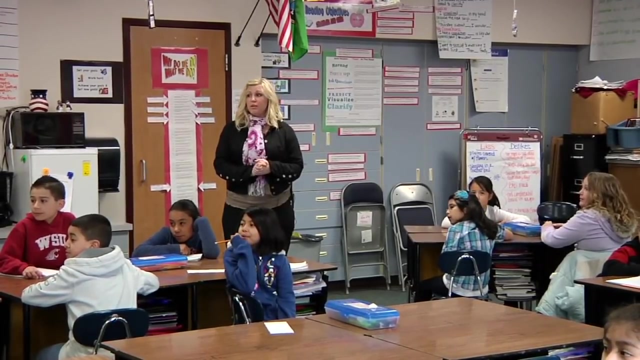 We're going to do a review lesson today for our test. boys and girls. I will apply what I have learned about expressions, equations and patterns to solve problems. I will defend my answer. I will defend my answer To my group, To my group, Using words, numbers. 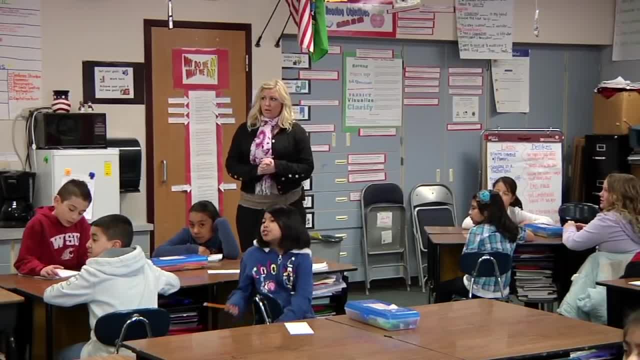 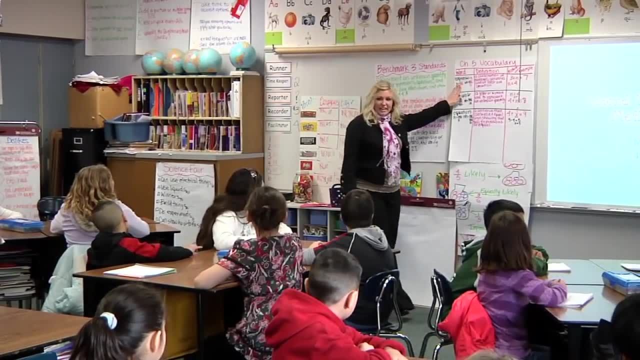 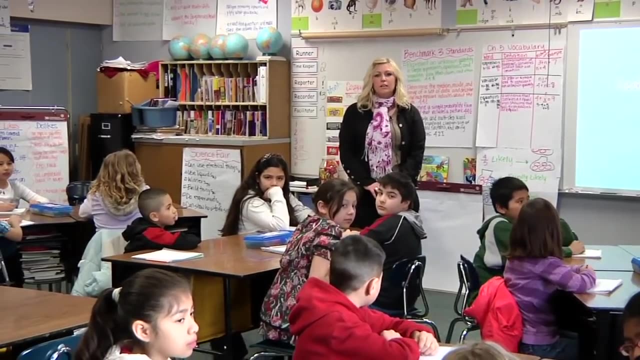 and pictures Using words, numbers and pictures. Okay, so we talked a lot about expressions, variables and equations. this lesson: Who remembers what an expression is? Who remembers what an expression is Jill? Um, it's a problem with like a letter in it. that's five times. 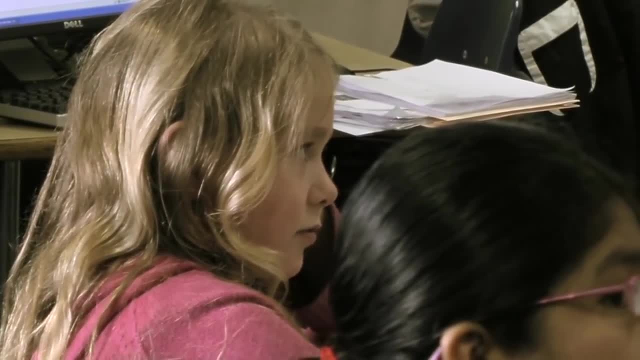 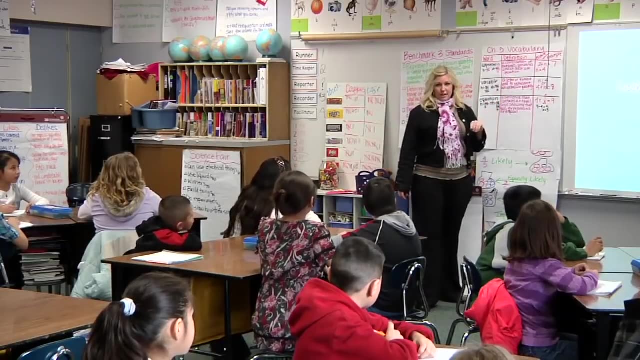 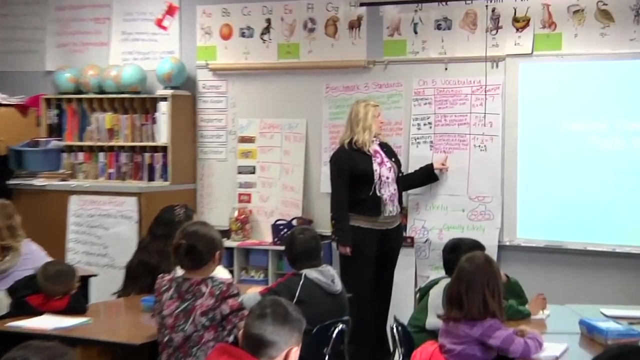 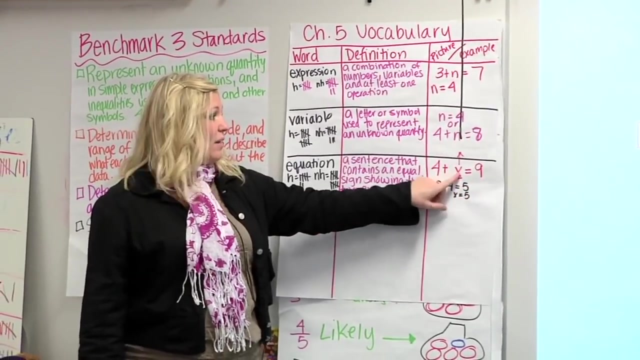 e equals Okay. alright, so it's a problem with a letter in it, but it doesn't have an equal sign, right? An equation is a sentence that contains an equal sign showing that two expressions are equal. So four plus x equals nine. Did everybody remember that? Okay, and x is called. 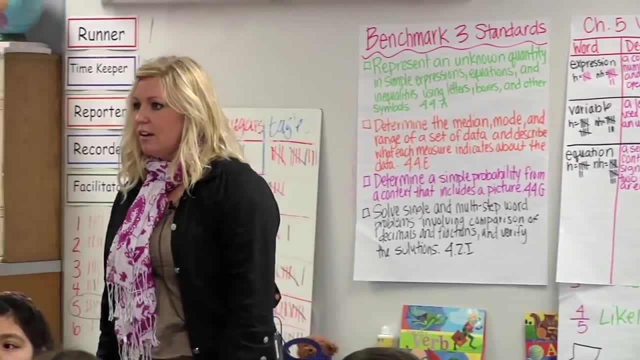 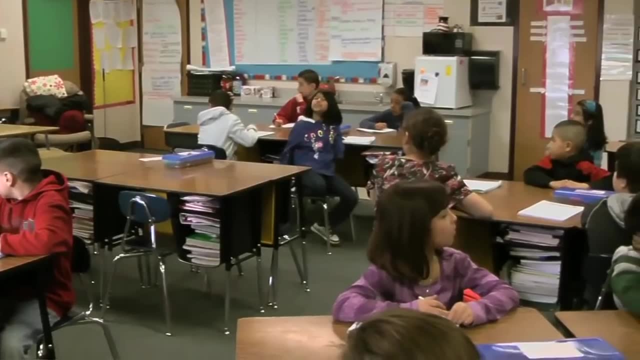 a what? What is x called Isaac? A variable? A variable, Very good, Okay, so we're going to use the math. Okay, so today it says I'm going to defend my answer to my group using words, numbers and pictures. Who can explain to me how I do that? How do I defend my answer? 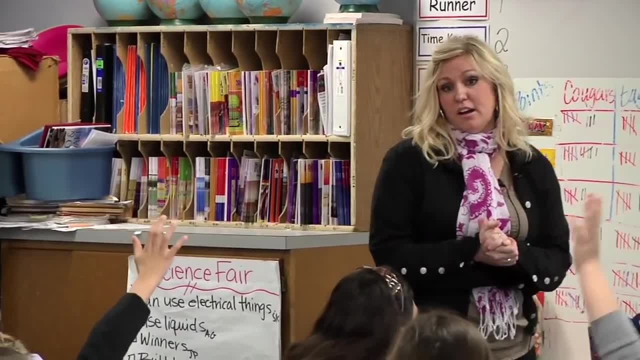 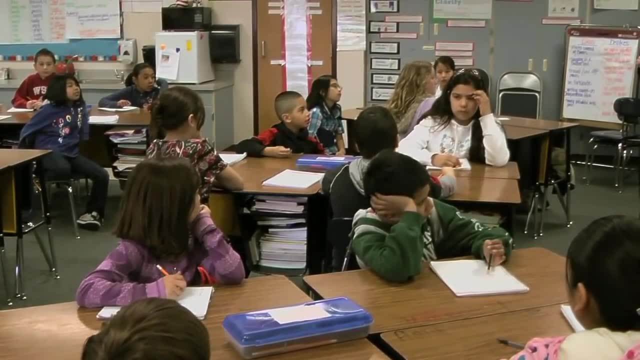 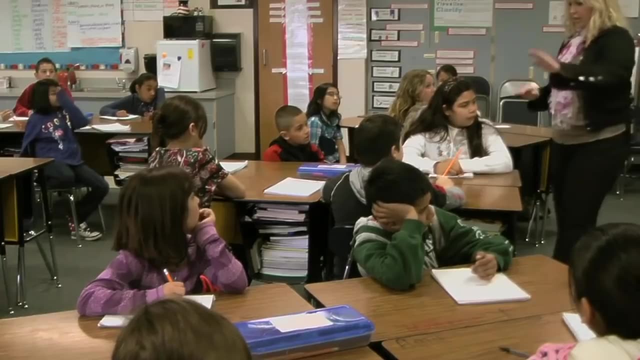 to my group. Do I just yell out the answer I got? What do I do, Alex? You start with one, two, three and four and you tell them and explain them: like what? how do your answers go? Okay, so Yesenia is a one, Jay is a two, you're. three and Ashland's a four. So does Ashland go first? Yesenia's a two, you're three and Ashland's a four. Okay, so does Ashland go first? Yesenia's a two, you're three, and. 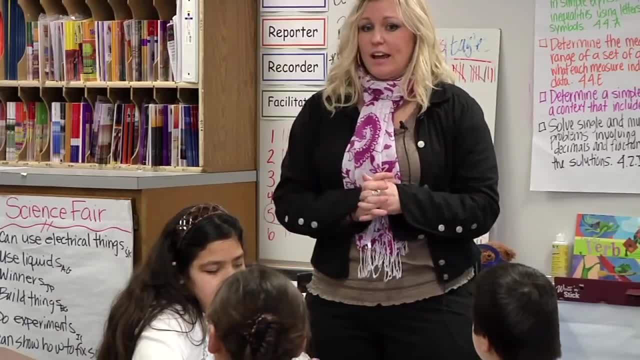 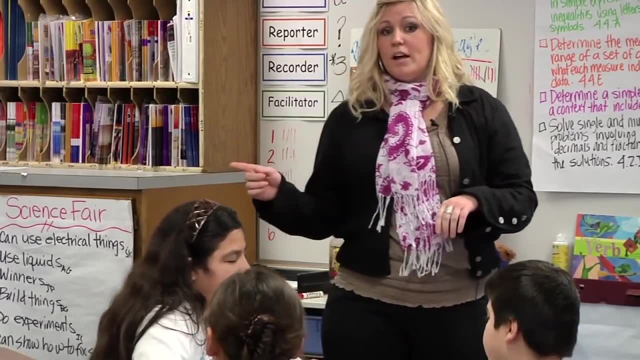 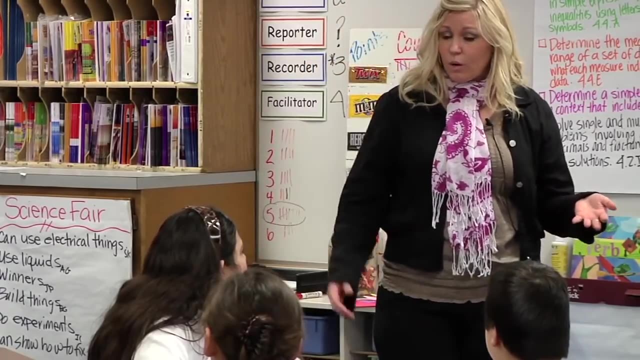 does Ashlyn go first? No, Yesenia goes first And does she just say I got five? No, she has to explain her answer. She has to explain her answer and show her work to you, right? So once you defend your answer and three of you have it right and one of you has it wrong, what do you do, Alyssa?